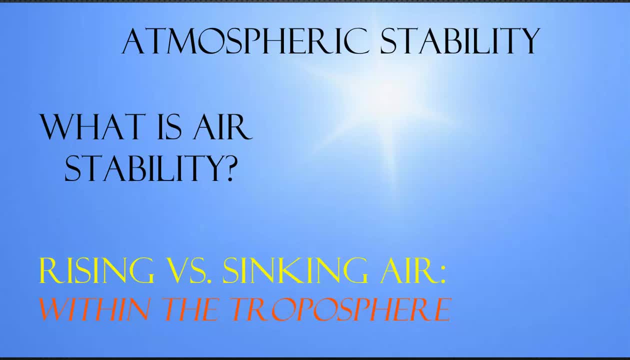 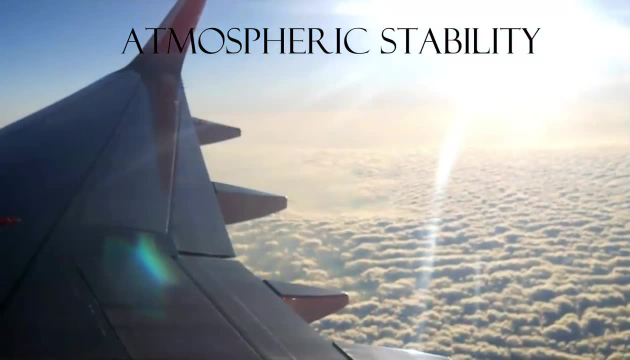 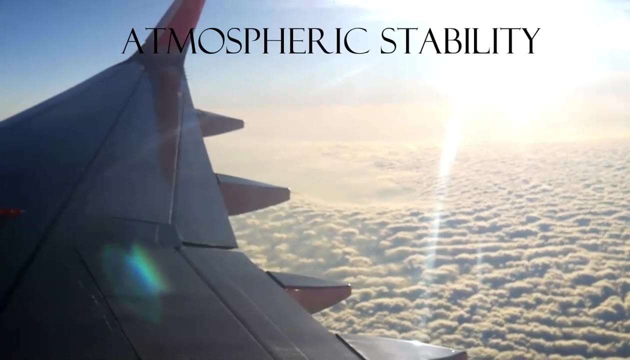 we've got to understand what's called stability and what air is doing. Is it going to rise, Is it going to stay in one place for a short time, Is it going to sink, And what this means for the conditions in the atmosphere and whether it will cause any kind of weather or be blue skies or. 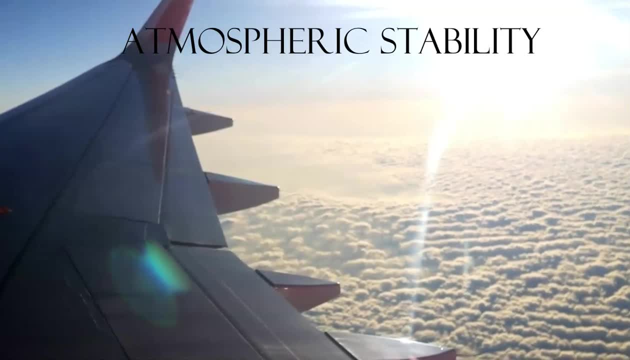 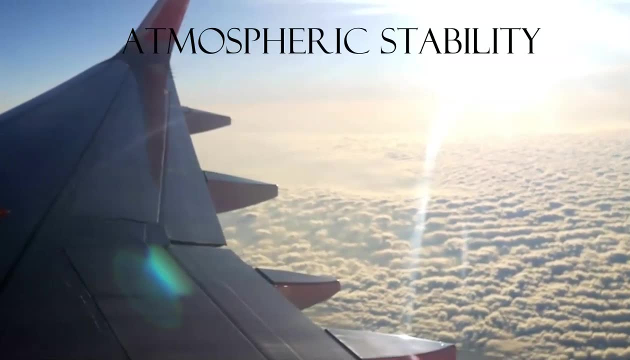 what kind of clouds are formed and if there's going to be some sort of precip in the near future. So weather forecasting and travel like airplanes and hot air balloons is all related to stability of the atmosphere. So when looking at the stability of the atmosphere, 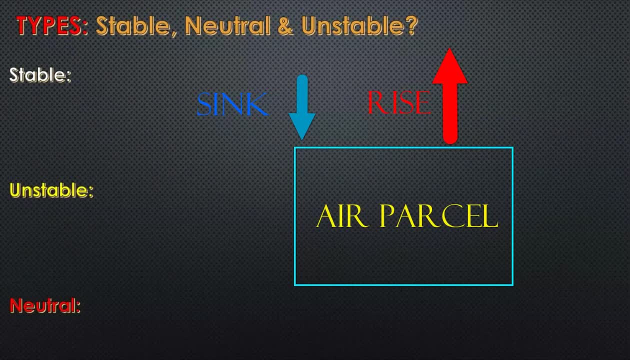 we're looking at the air parcel. What's the air parcel going to do? Is it going to rise, Is it going to sink? It will stay at the same altitude And this is based on the heating and cooling of the atmosphere. So we measure the air temperature at a certain altitude. These are consistent in. 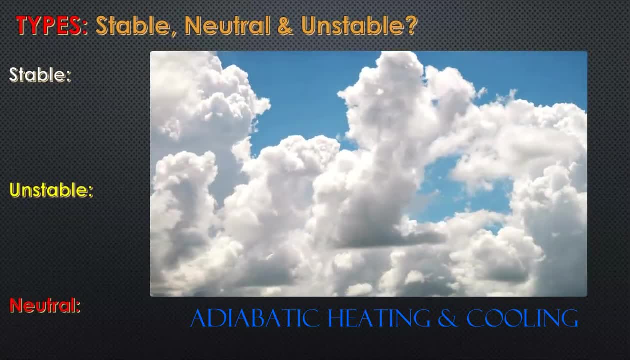 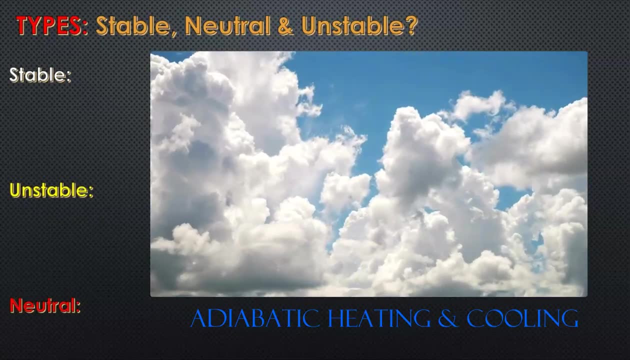 terms of the temperature of the earth. So we're discussing the adiabatic heating and cooling. We're looking at the air parcels temperature at certain altitudes and how this relates to the environmental lapse rate, And there are three types of stability in the atmosphere. There is 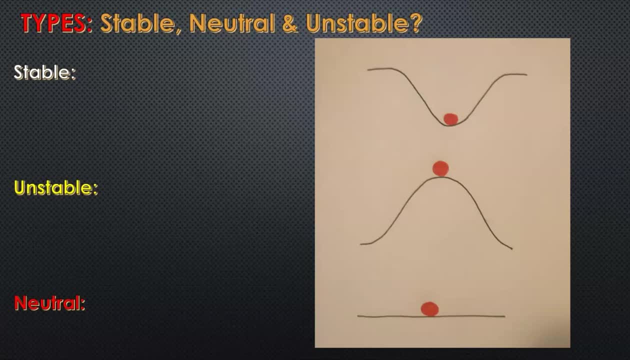 stable, unstable and neutral. Now the air parcel can go through different phases, where it can be stable and then become neutral, or even become unstable, based on different conditions. Now this diagram is showing you a very, very basic understanding of these terms. So the top 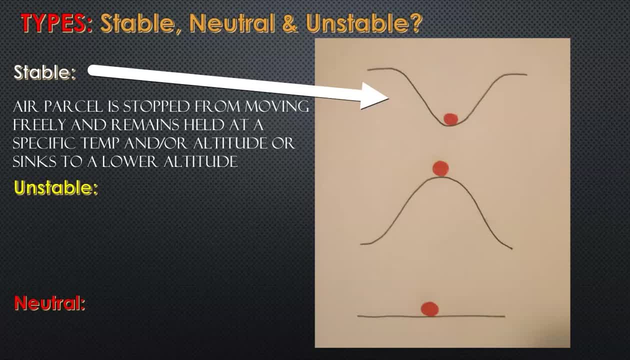 diagram which is stable. it shows how the air parcel in the atmosphere, namely the troposphere, is going to stay at the same altitude. It will try and move, but it's kind of stopped, or even sink down to a lower altitude based on conditions. So stable is where you'll have it: either sinking, 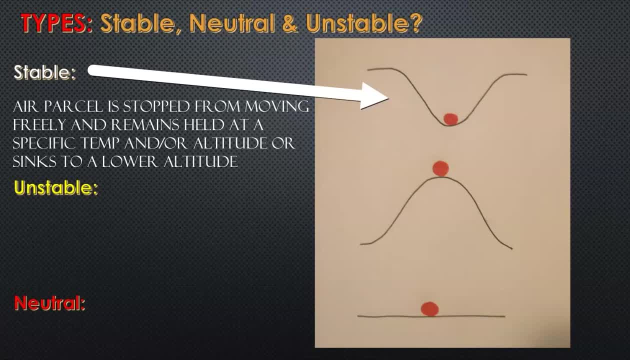 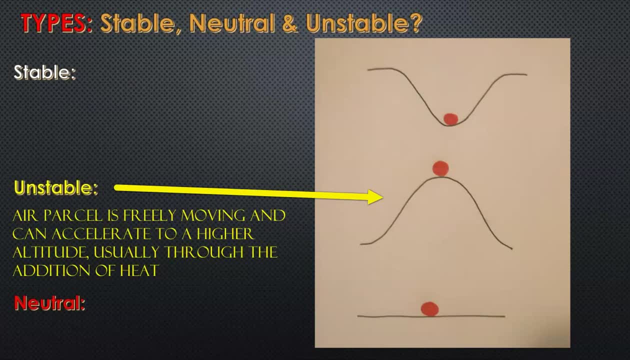 or you'll have a continuously the same altitude of the air parcel compared to unstable, where this air parcel is likely to be pushed out of the altitude and forced to accelerate to a higher or increased altitude due to, for example, the addition of thermal energy and hot air is going to rise. So this 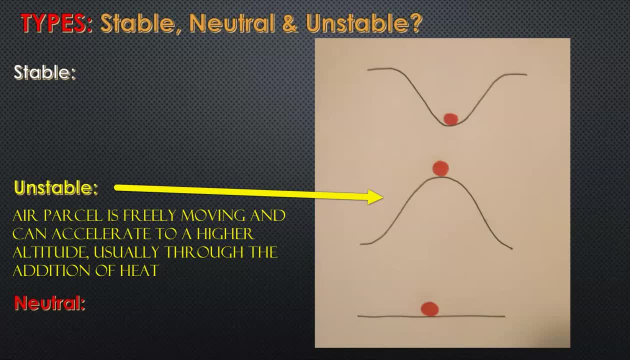 this air parcel become unstable when it is forced to rise up through addition of heat or forced to rise through addition of a cold air mass, and it's forced to rise up higher. So this air parcel will accelerate up and decrease in temperature as it increases with altitude, And this also 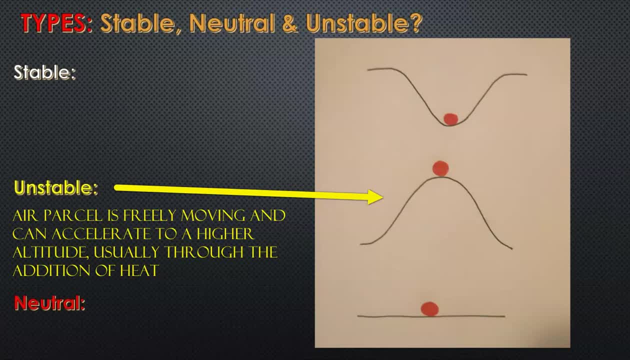 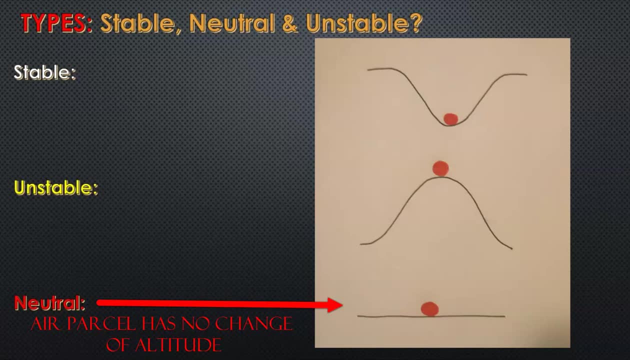 looks at strong addition of thermal energy, or a lot of thermal energy added. Then we have neutral. Neutral is rare in the atmosphere to have a consistently neutral air parcel. However, it is a point that's in between stable and unstable, where there's 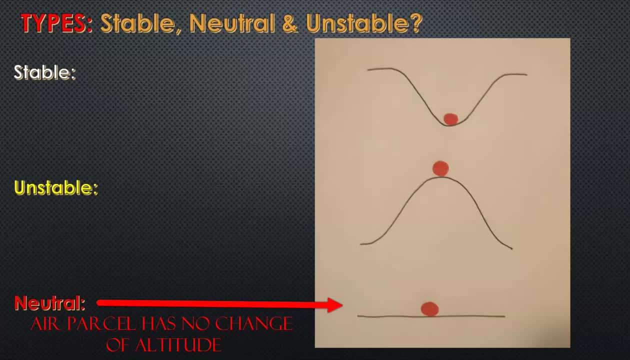 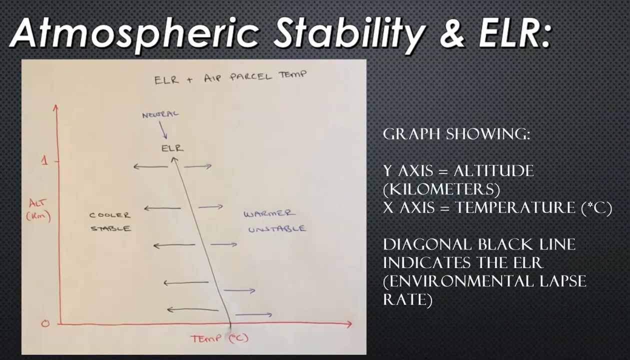 a conditional situation, Based on a short time, of the air mass or the air parcel not being stable or sinking and not being unstable and rising. So this diagram looks at the combination of this atmospheric stability with the environmental lapse rate. Now on this diagram again, I've gone a one kilometer or. 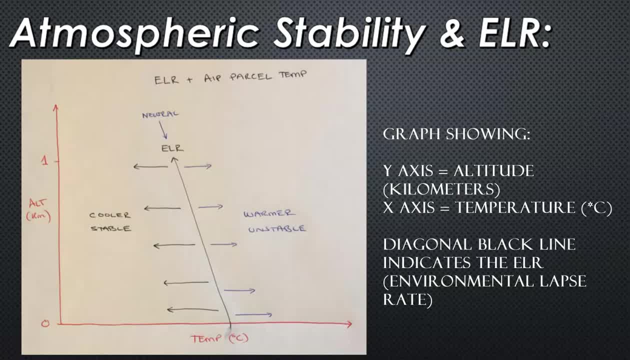 1000 meter altitude on the y-axis. On the x-axis we have our temperature in degrees Celsius. So I had this black line, diagonal black line, showing the ELR. Now I haven't any numbers on the bottom- which basically means that this is a generic lapse rate for the. 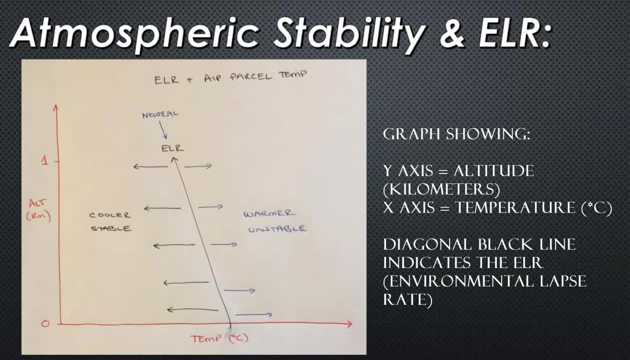 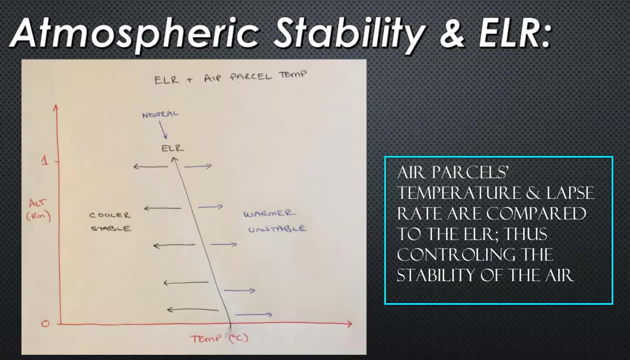 environment and the air parcel, which is going to be a different temperature in theory to the ELR. Now, if it's the same temperature, it would just be moving higher in altitude and decreasing at the same lapse rate as the ELR. That will be a neutral environment or atmosphere. However, 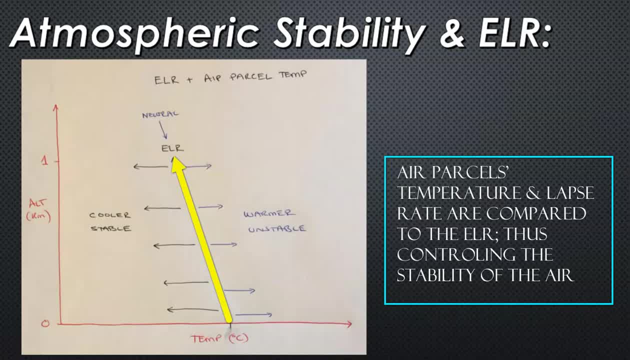 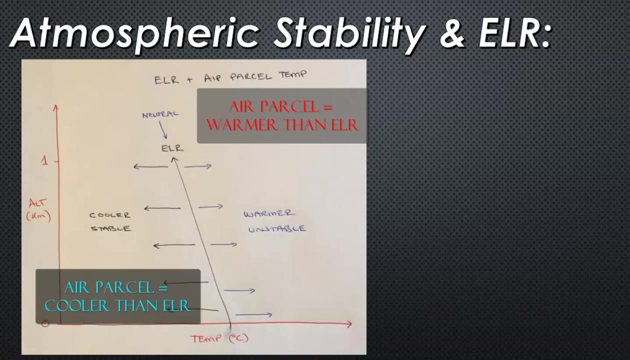 if the air parcel is of a different temperature and lapse rate, it would start at the same temperature as the ELR at the surface. However, because it's a faster or slower lapse rate, it would either cool down faster or cool down slower than the ELR. 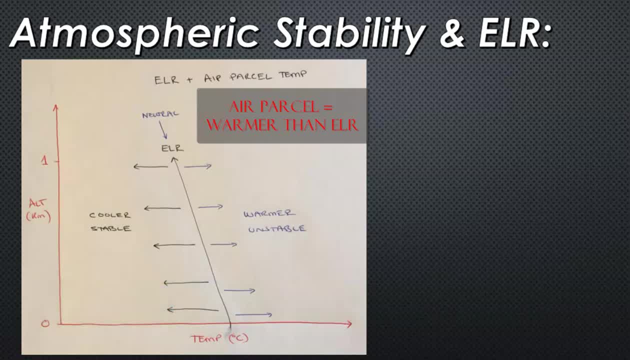 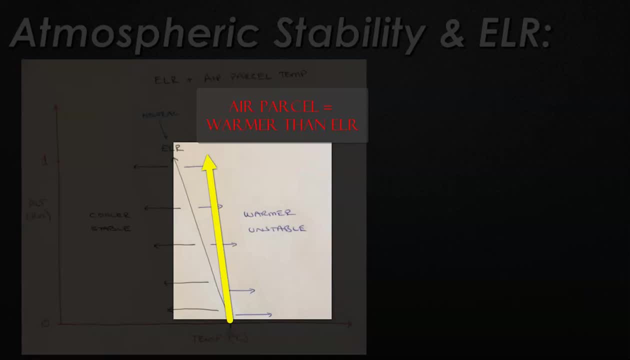 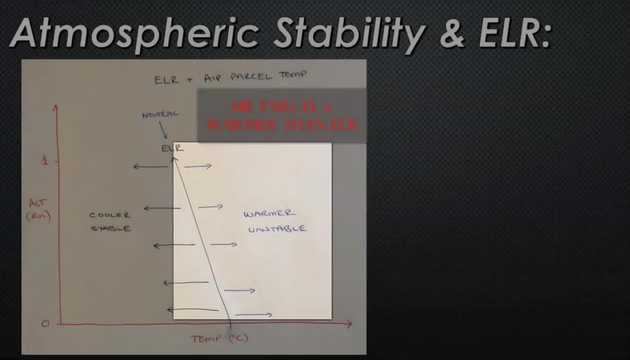 For example, if the air parcel was to cool down slower than the ELR, it would fall on the right hand side and this would be classified as unstable because the air is still warmer in the air parcel at a certain altitude compared to the ELR or the air around the air parcel. On the other hand.